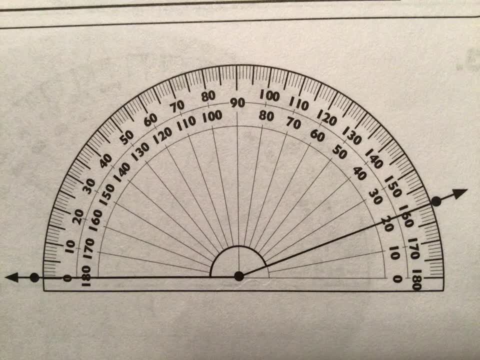 small group sessions or the small group session, it was apparent that maybe I needed to do a little follow-up on this. So when we're thinking about inner scale and outer scale, one of the things that was helping the group that I was working with was to think about this protractor as 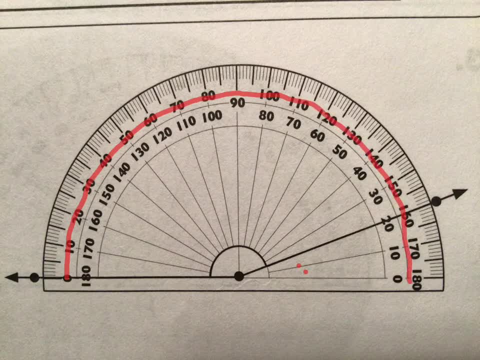 almost like a rainbow. So you know how rainbows: the first color is red, and then we have orange, yellow, green, blue, purple. right, We're just going to deal with the red and the orange. So if from the 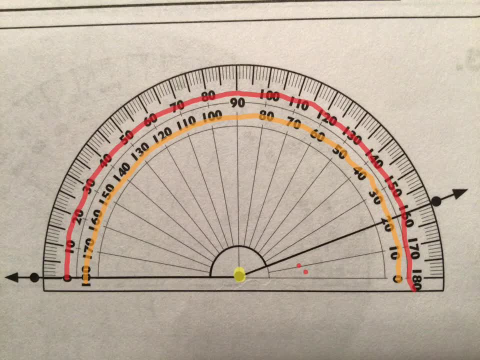 center point. okay, there's the center point. yellow From the center point. the inner scale is going to be orange. It's closest, it's on the inside, to the yellow dot and the red is the outer scale. okay, It's outside, oops, outside the inner scale. So that color coding. 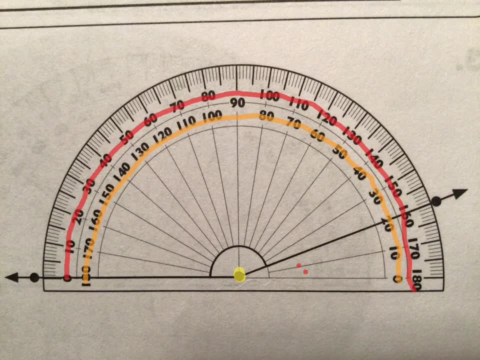 really helps Some students to see okay inner scale. those numbers going around in the orange are part of the inner scale and the numbers in the red are the outer scale. So that might be a tip that helps some of you. In fact, with some of the students I was working with, we even said: 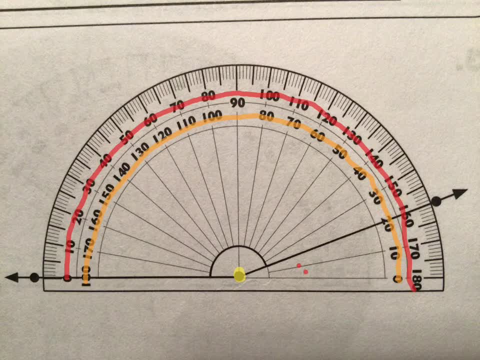 get a red and an orange crayon and just color code your protractor so that you can see: okay, am I using inner or outer? And then just a reminder: how do you know if you're using inner or outer? Well, if you look at the ray that's drawn and lined up with the 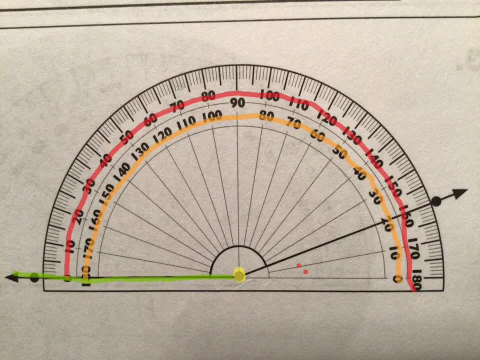 baseline. if it passes through zero on the, where's my pointer? There we go. If it passes through zero on the outer scale, you're going to use the outer scale to measure that angle. Okay.